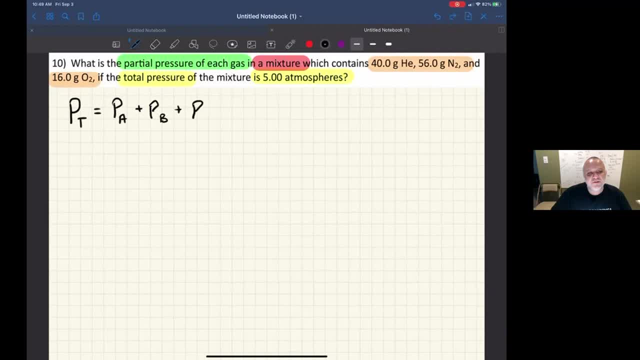 equals the partial pressures of each component. Now, the reason that I write this down is to give some grounding on what the partial pressure is. now I can write that the partial pressure of a component is equal to the mole fraction of that component times the total pressure. Now recall: 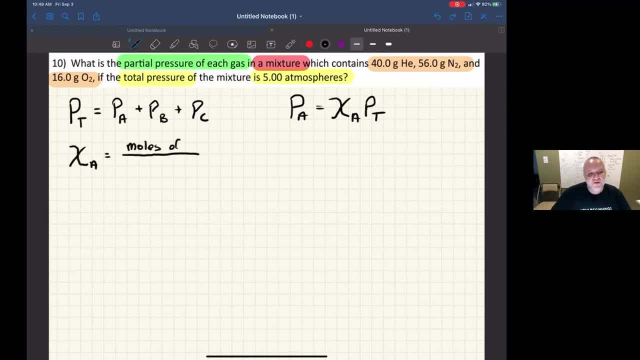 that the mole fraction of a component is equal to the mole fraction of that component times the total number of moles, And so with this information I can start to attack this problem. So what I need to know is the moles of each component. So I got a little bit of work to do in converting grams to 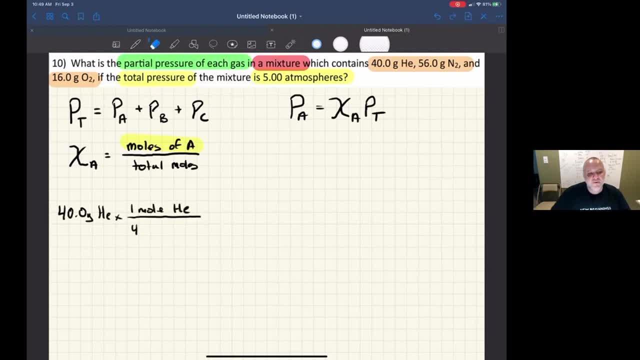 moles, So 40 grams of helium divided by its molar mass. I also need to do the same thing with nitrogen, And so I've got a little bit of work to do in converting grams to moles, So 40 grams of. 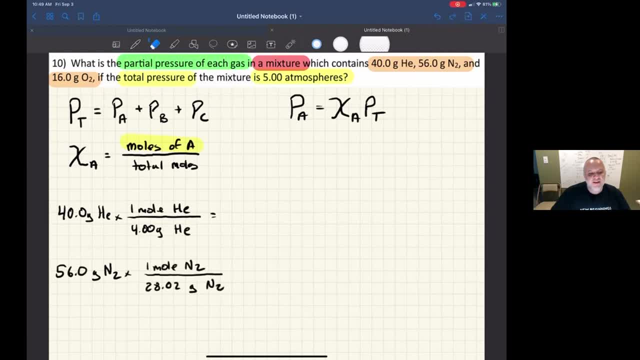 hydrogen divided by its molar mass, And I need to do the same thing with oxygen divided by its molar mass. When I put those into the calculator, I get 10 moles, 2 moles and 0.5 moles. Now let's. 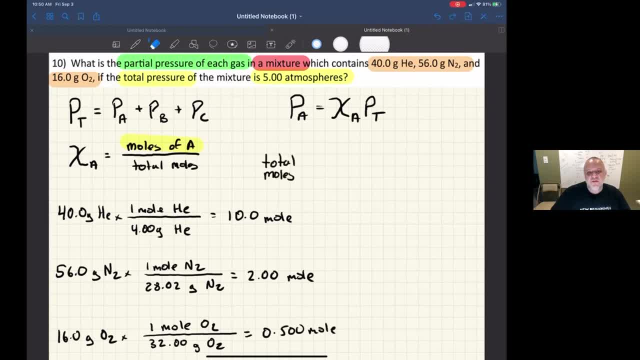 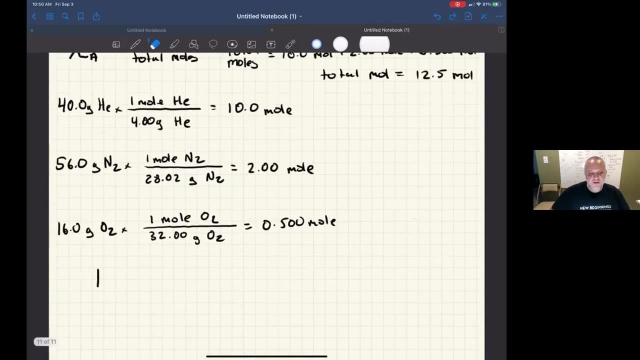 figure out the total number of moles. The total number of moles is going to be 10.0 plus 2.00 plus 0.500.. And so I get 12.5 moles. Okay, So I've got some work to do now to figure out these partial pressures. Now let's write those. 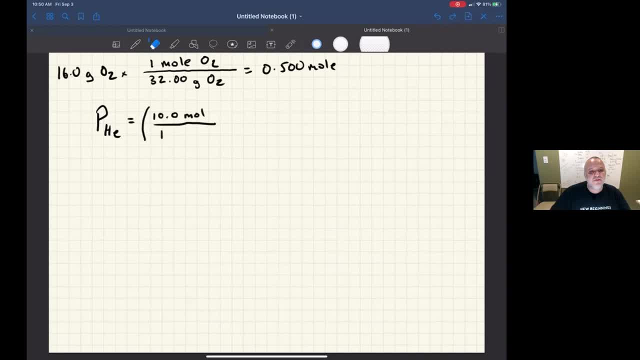 formulas down. The partial pressure equals the mole fraction. So that's the mole of the component divided by the total moles. And the moles of helium were 10 divided by 12.5.. That's the mole fraction for helium times the total pressure. Now let's do the same thing for nitrogen. 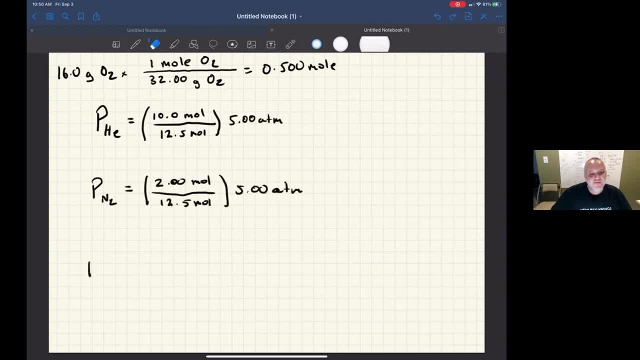 That was 2 moles divided by 12.5 moles Times 5.. And for oxygen it's 0.5 divided by 12.5 times 5.. So let's get our calculator out and work on that, Okay, The mole fraction of helium will end up being 0.8.. And 0.8 times 5 is 4 atm.